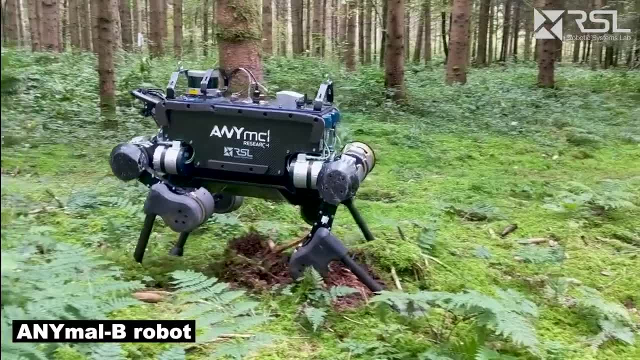 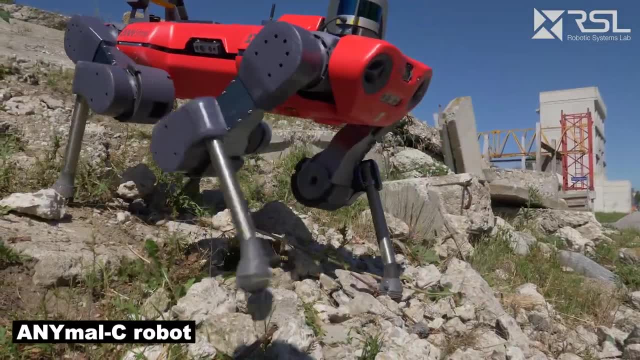 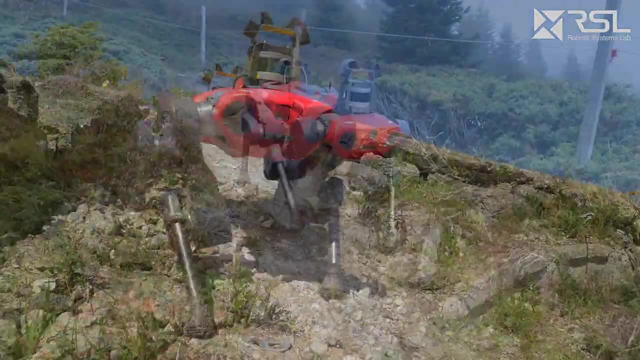 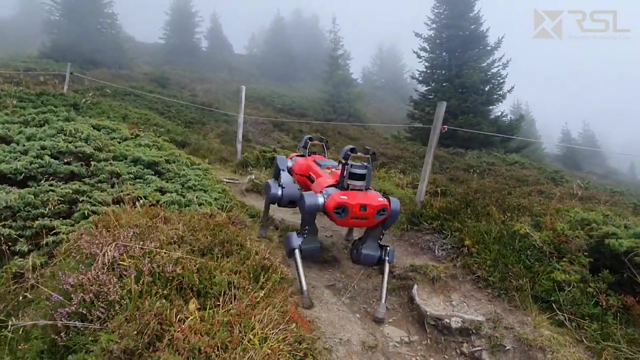 Without any real-world data or accurate terrain models. the control policy is robust in natural environments with highly irregular terrain profiles and unknown physical properties such as friction and compliance. To evaluate robustness and generalization, we tested under various conditions and with different robots over the time frame of more than half a year. 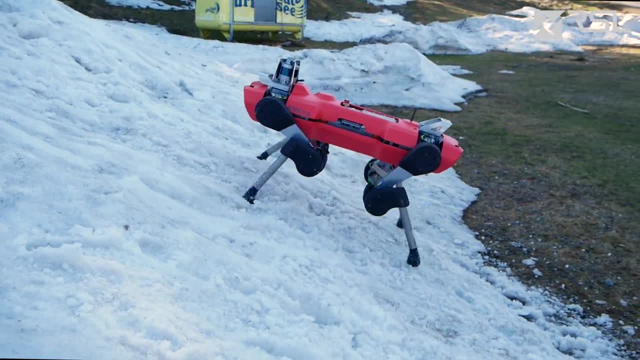 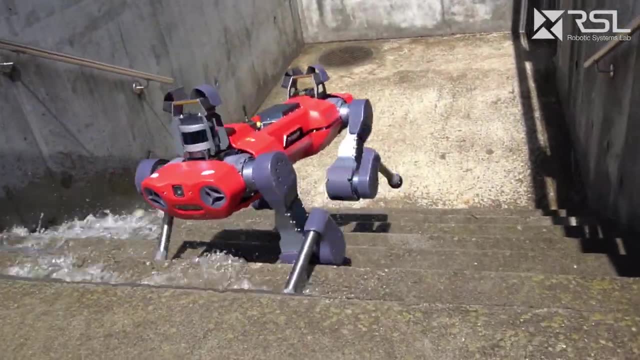 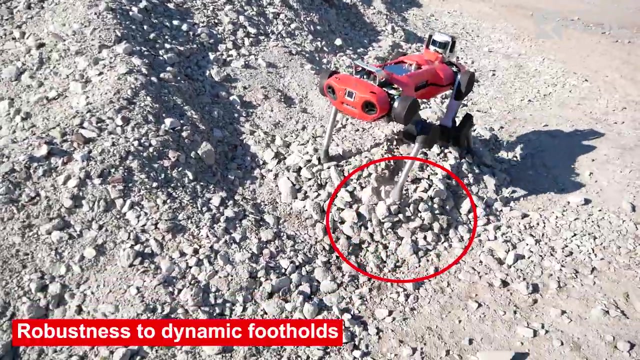 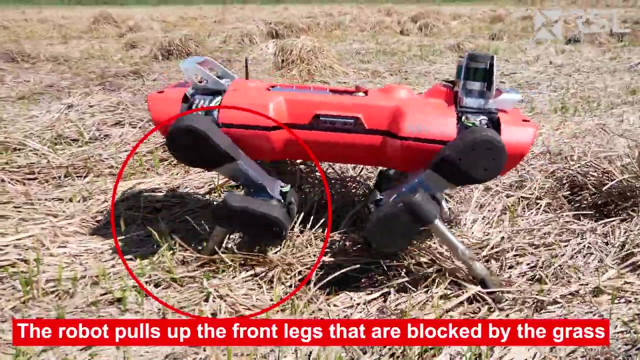 The proposed method does not use cameras, LiDAR or contact sensor information, but only relies on proprioceptive sensor signals to adapt to diverse terrain conditions. The controller can handle dynamic footholds, remains robust even when the robot's feet are impeded, and successfully handles significant disturbances. and 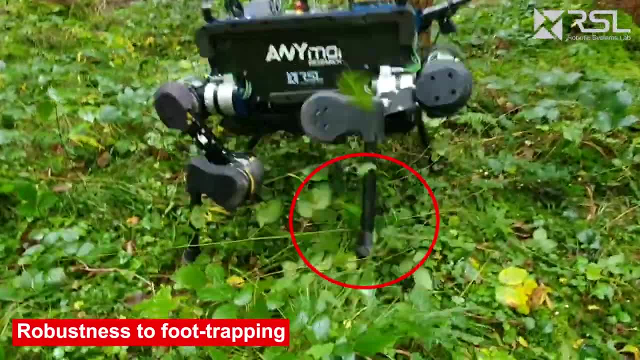 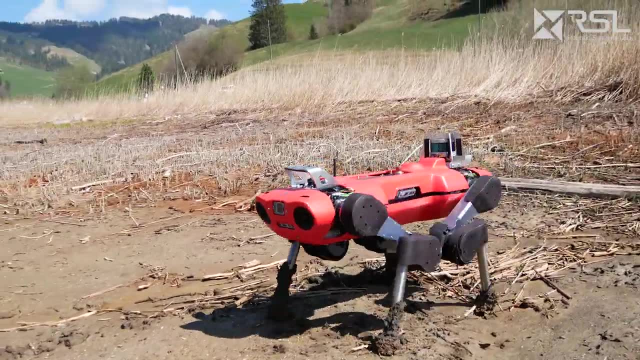 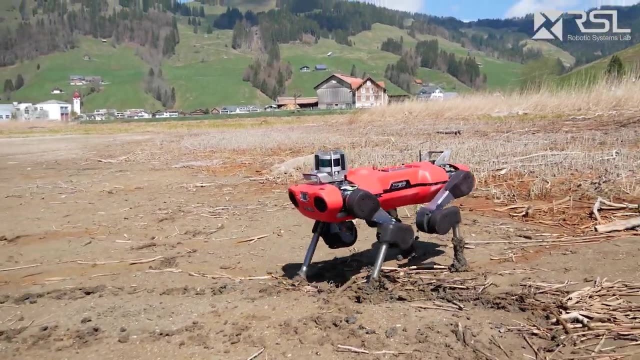 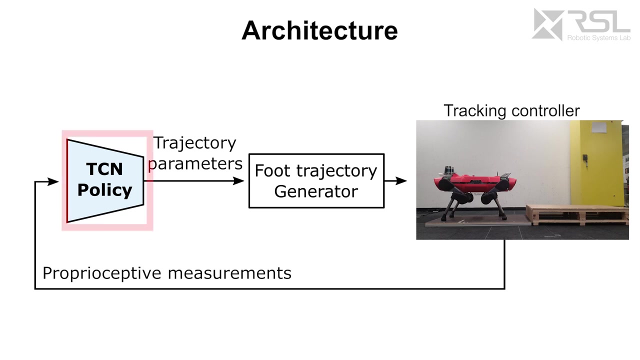 changes to the robot's legs, which are often present when walking through vegetation. In fact, our system was able to traverse any terrain shown in this video without a single fall. For each robot, the same controller was used in all environments and conditions. Here is the structure of our controller. 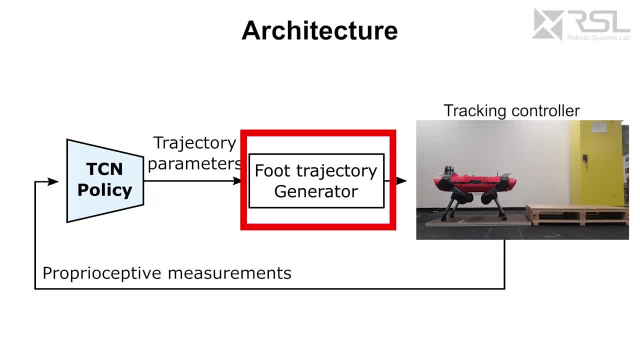 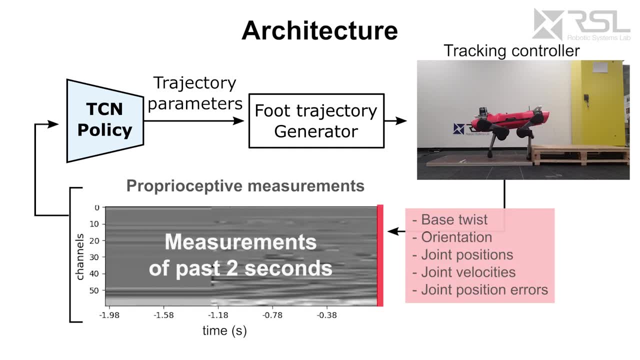 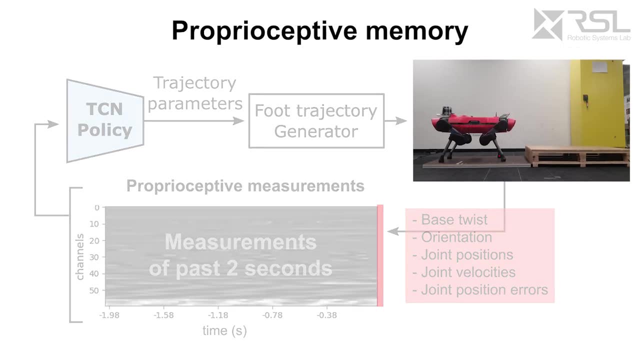 The controller is based on a temporal convolutional network policy that modulates the robot's feet trajectories. The policy acts on a sequence of proprioceptive measurements, which are provided by an inertial measurement unit and joint encoders. By analyzing two seconds of proprioceptive history, the policy can identify different. 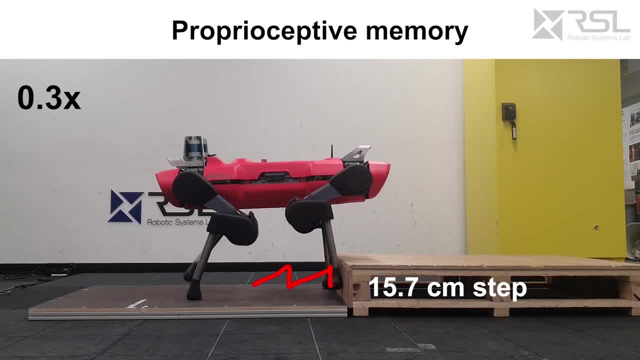 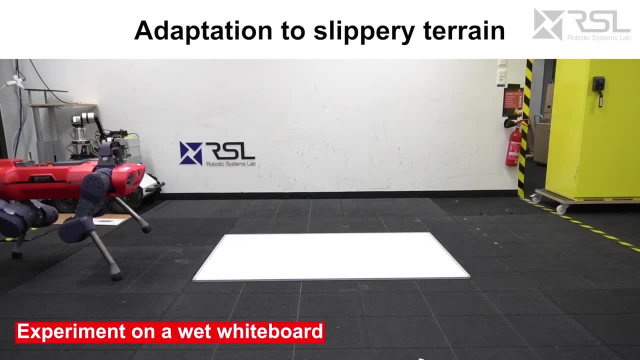 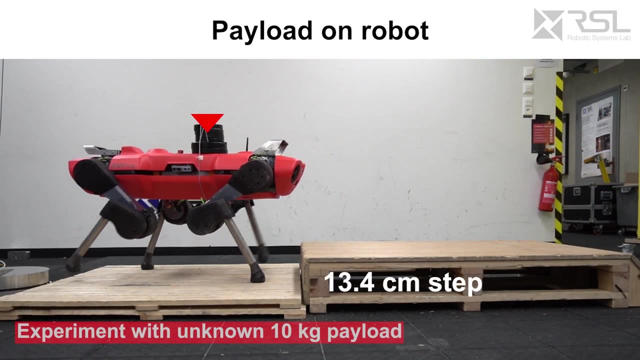 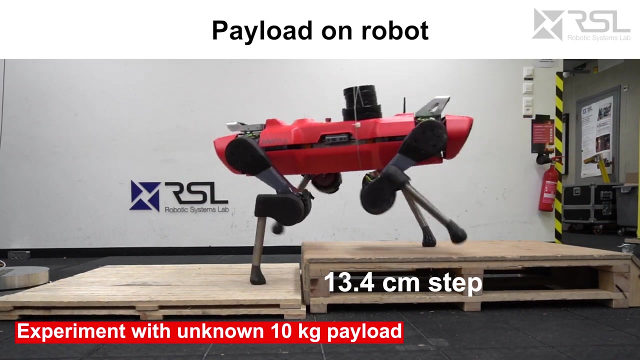 events like this collision with a step and adapt to different terrains and disturbances. Our controller can adapt quickly to changes in terrain properties and maintain a consistent stability. Since we apply random disturbances during training, our controller can robustly handle large model inaccuracies like unknown payloads. 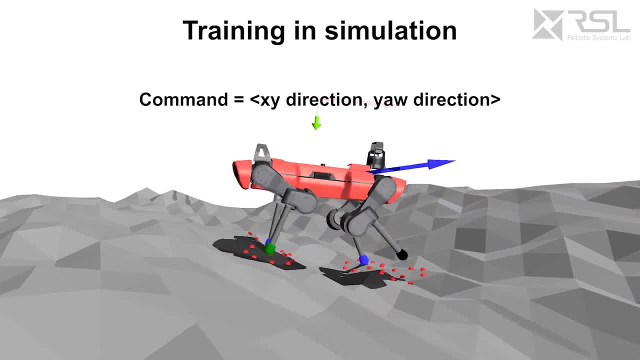 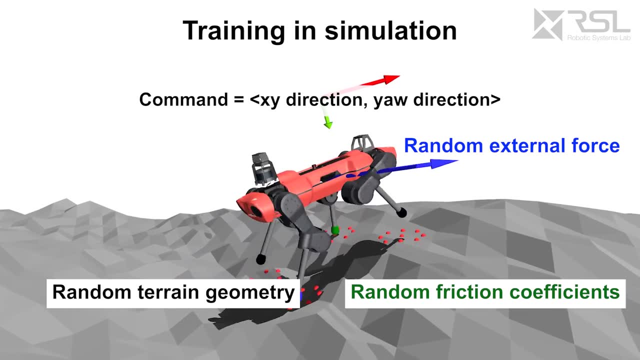 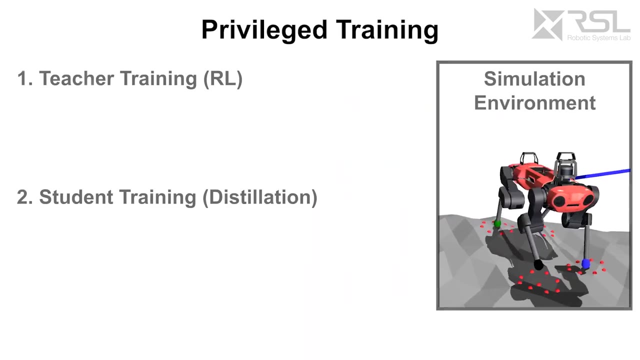 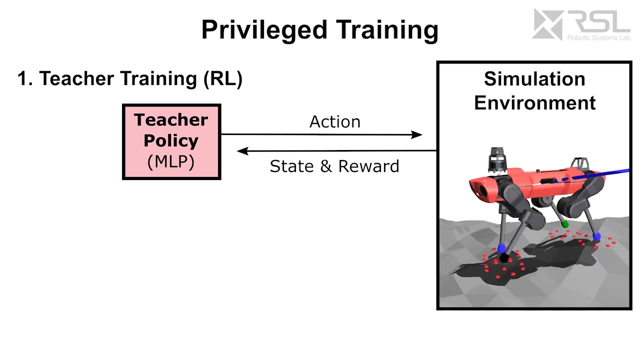 The control policy is trained in simulation to follow a command direction on rough terrain. In every training episode a new environment is synthesized and external disturbances are applied as the robot learns to remain stable and maintain the desired heading. Training is done in two steps. We first train a teacher policy that has access to